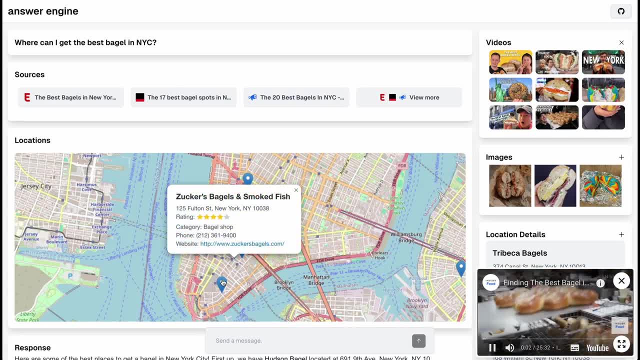 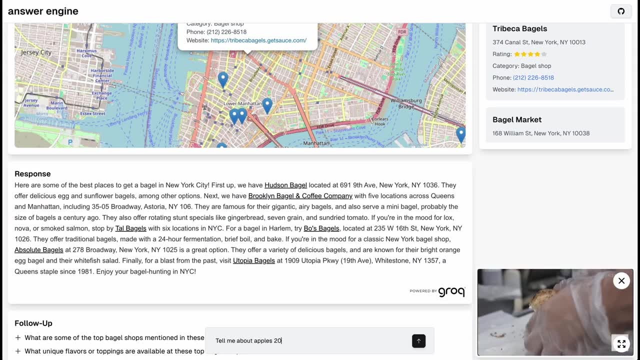 In this video, I'm gonna be showing you how you can set up your own conditionally rendered UI based off natural language by leveraging the new croc function calling capabilities as well as the Vercel AI SDK. I'm going to be going over three different examples. 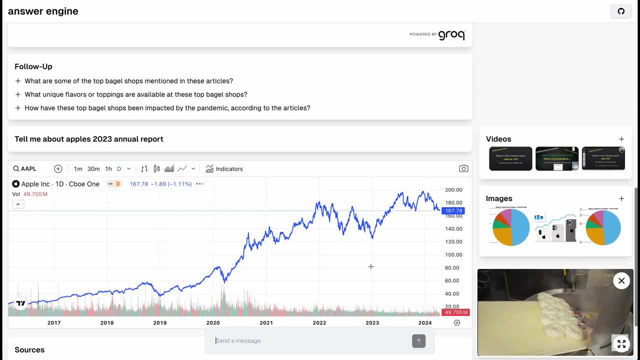 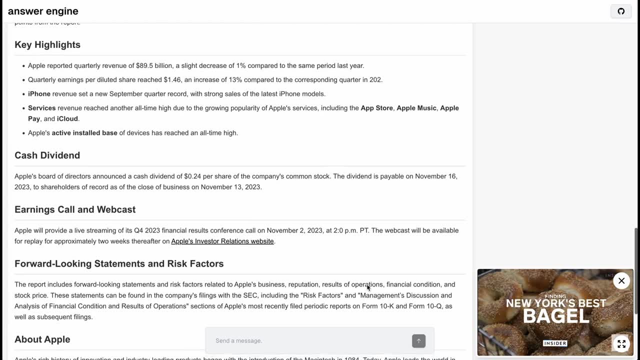 I'm going to be showing you how to set up a map with different locations by leveraging the server API, and be showing you how you can set up a stock chart that's interactive from TradingView, which is completely free, and be also showing you how to set up a simple shopping component. 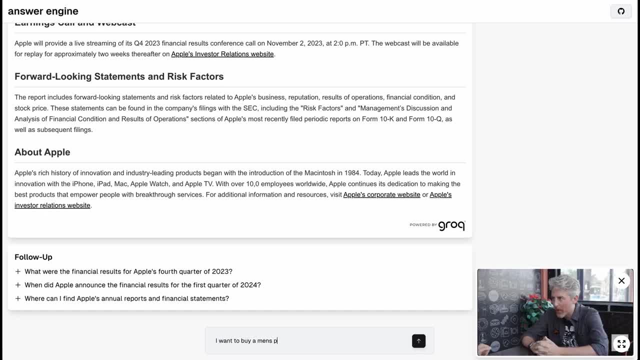 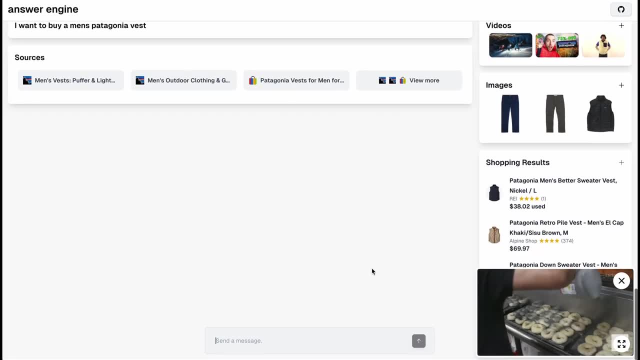 So if you didn't see my previous video where I built out this answer engine, this is really building off of that. I just genuinely want to thank everyone for their support over these past few weeks. This repository really took off in a way that I was not expecting. 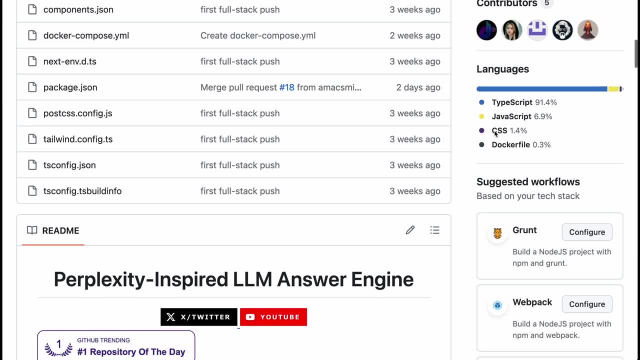 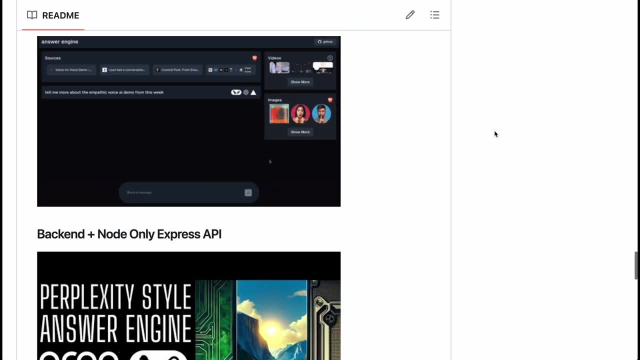 I've had different creators create content about the video which is hard to believe. I've had, all of a sudden, different companies reach out to me. I'm just glad that I'm able to provide something useful where it's, something that either you can build with or learn from you, just like using the. 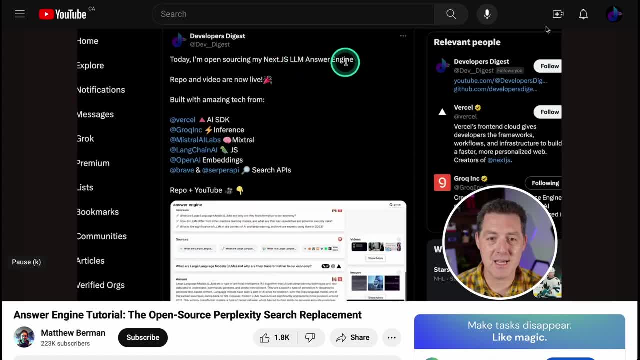 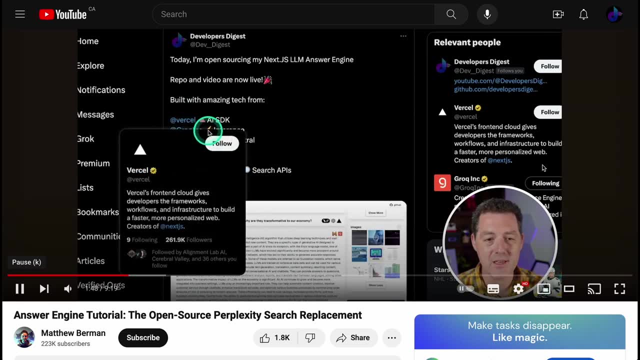 tool I'm playing right now for the product. I'm going to be showing you how to set up a map. I'm going to be building out some features that I haven't yet seen in any sort of other chat interface yet and show as examples. I'm just excited to see where this project will go Now. 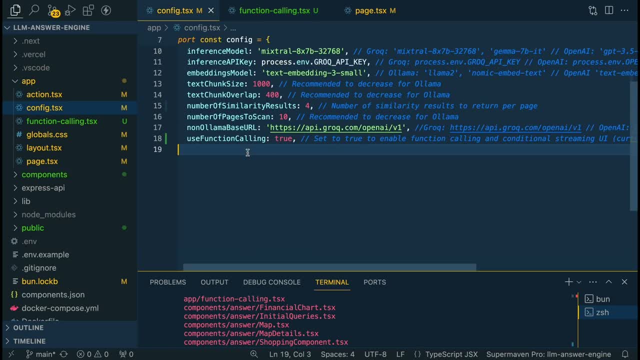 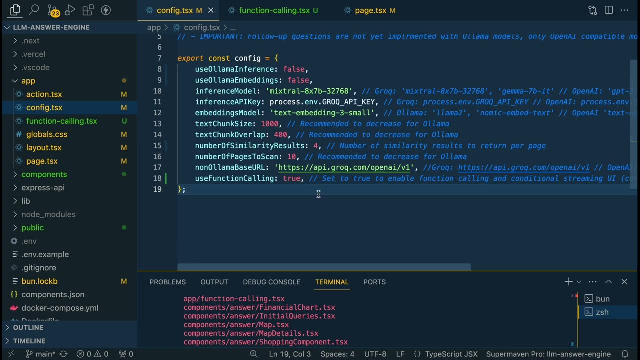 the first thing that we're going to do within our project. we now have this configuration file, which I have commented galore here. the first thing that we're going to do to set up this new function calling capability is we're going to set up this key value pair within the configuration. 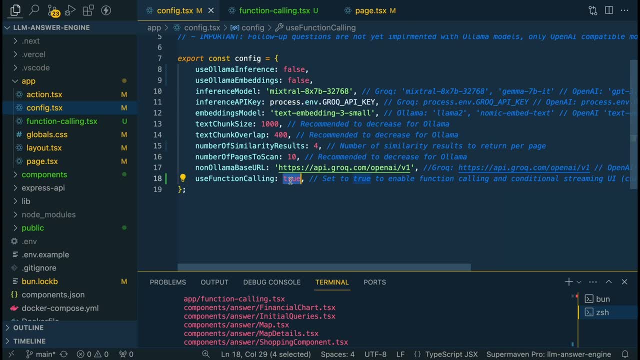 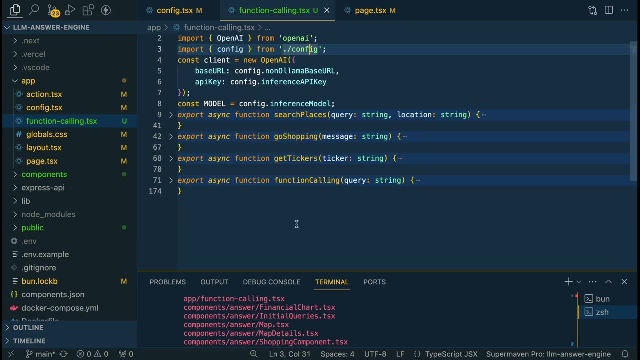 object. I have this key of use, function calling, and you can simply turn it on or off, And then, adjacent to the action and config, we're going to make a file called the function calling. Right now I'm going to put all of the functions as well as the logic that orchestrates. 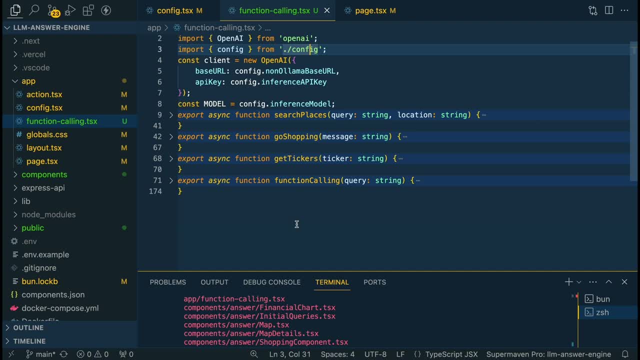 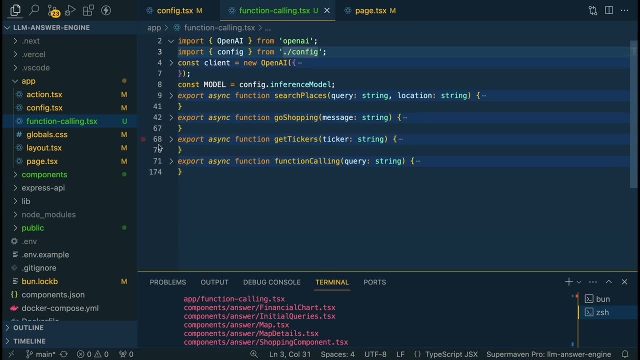 the function calling capabilities from the LLM all within one file just to show you for demonstration sake. we're going to be using the open AI SDK. I still have it set up to croc, So we are going to be using that new croc function calling capability If you do want to use. 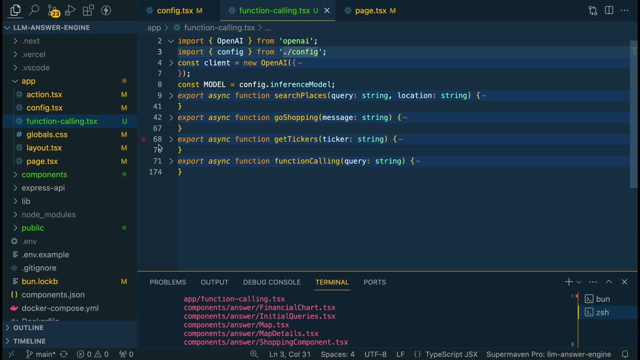 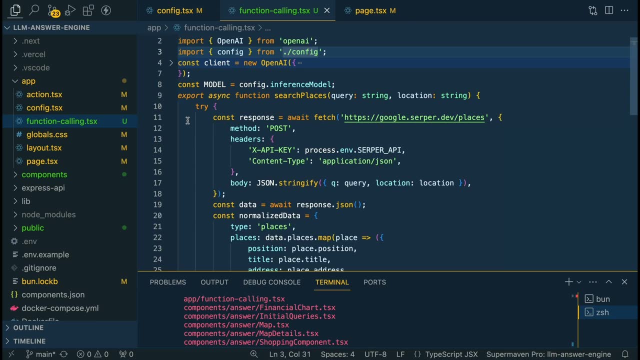 something like GPT 3.5, you can use that as well. What we're going to be doing is we're going to be using three simple functions, And the thing with these different functions is if you want to swap these in for some of the components that already exist, like the images component or the videos. 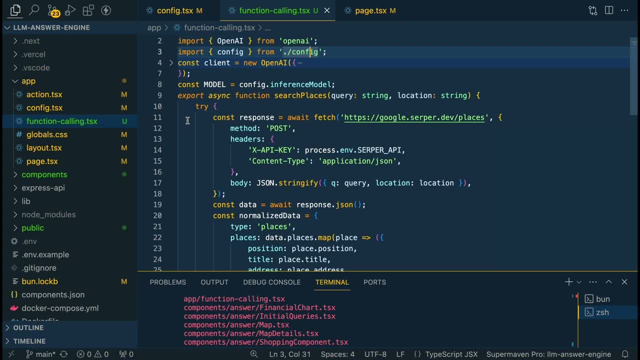 component. So let's say you don't necessarily want to always render images or videos. you could just throw them in here and have that logic be conditional. The first function that we're going to be setting up is the search place function. The end state of this is we are going to have 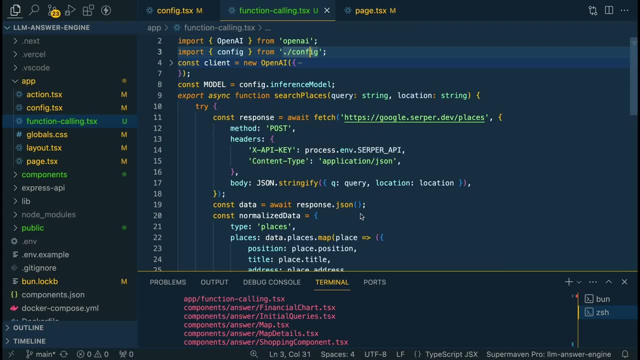 an interactive map that we can use the map itself. we're going to be using leaflet, which is a source library- we don't need to pay for anything like a Google Maps API key or anything like that- And then we're going to be leveraging the already existing server API that exists within our 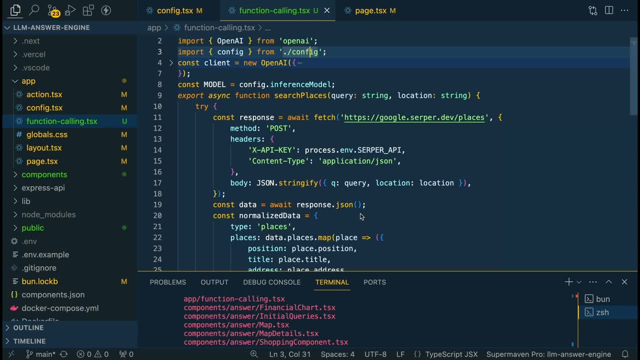 project. If you already have the project and you just want to bolt this on into the project that you already have, you can leverage those API keys that already exist. within our first function, we're going to specify that we want a query as well as a location, And this is going to be how. 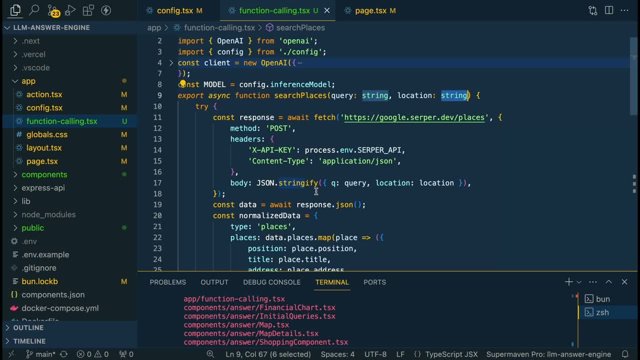 we render things like an Italian restaurant in New York or a bagel shop in San Francisco or whatever, or anything within this particular function. Within the function, we're just going to ping the Serper endpoint and we're just going to send in our API key, And then we're also going to be: 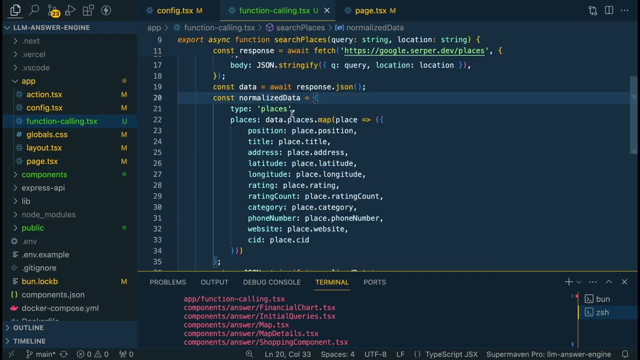 sending in that query and location that we had just talked about. Once we have that, we're going to normalize the data a little bit And then we're going to have this key of places. Now, the reason we're going to be doing this is going to be how we later route those different functions on where. 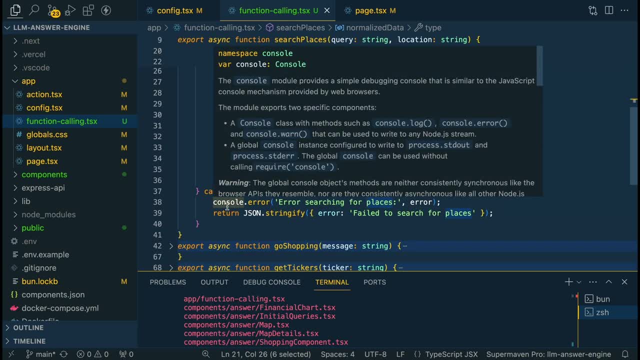 they need to go within the UI. Once we have that, we're just going to set up a catch if there are any errors when we invoke this function. Next, very similar to the previous version, we want to enter on the client server or the traffic server. So we're going to enter a by default and then we're. 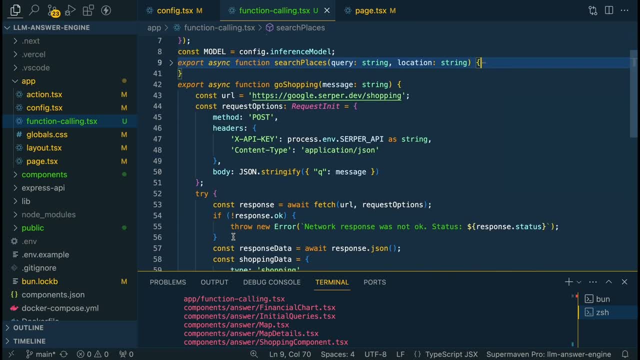 going to give it a password that the client server will be able to access in the future. And then we're Next. very similarly, we're going to call that server API to go shopping. if it detects that the user- quote unquote- wants to go shopping, we're going to specify: 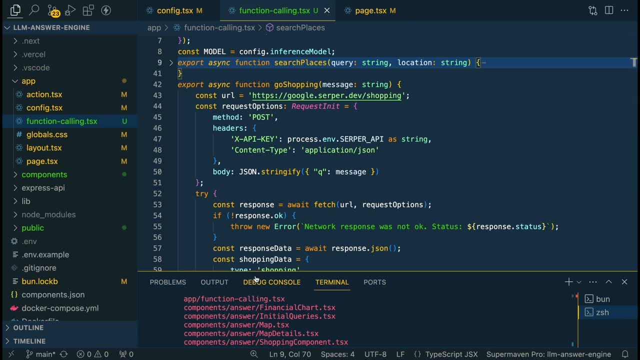 that we would need a string for this function, and then it's going to detect from the query on whether there's something like Patagonia vest or a boots or whatever you put in here- almost identical logic. we're going to be setting up the request the exact same way. 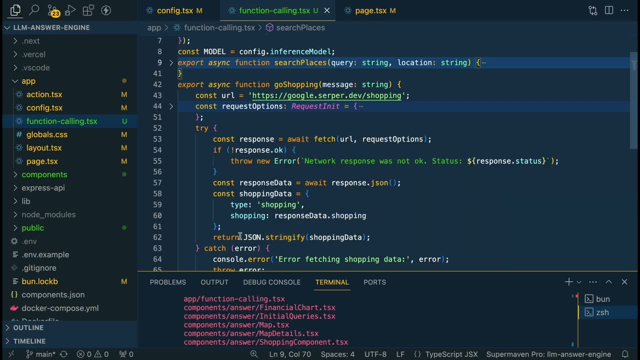 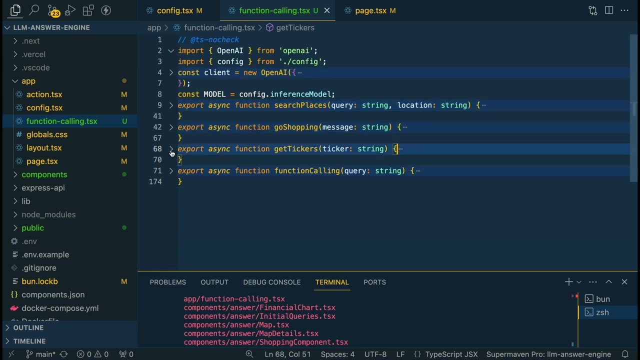 And then in this one, we're going to be adding that key of shopping, And then we're just going to be returning all of those results. Similarly, we're also going to log out if there are any errors when interacting with the API, and then in our last function, we're going to have a get. 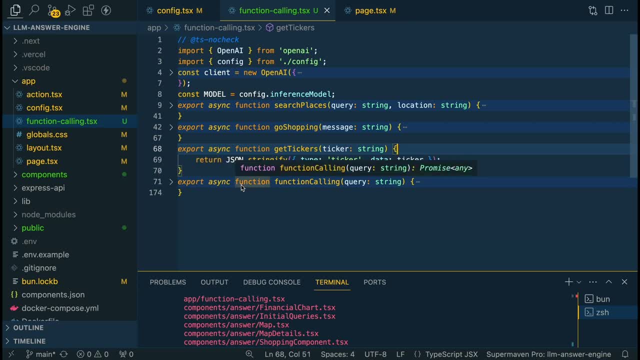 tickers function which is going to specify a particular ticker. So if we say I want to know more about Apple stock or Microsoft stock or whatever, it is all we're going to do within this is we're going to again add: 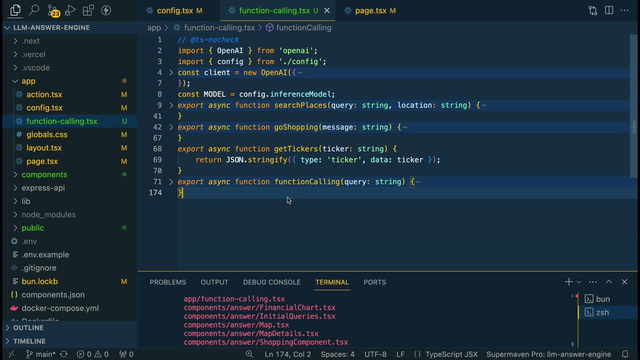 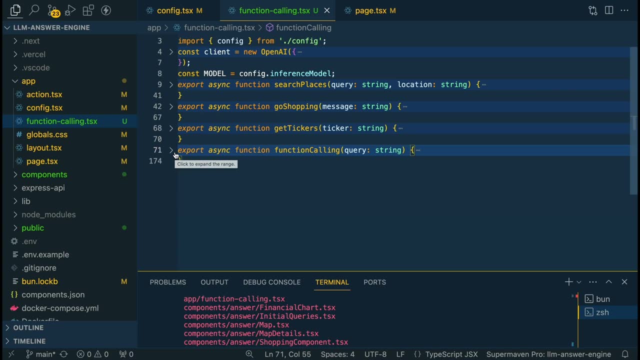 that key value, pair of type. we're going to specify that it's ticker and then we're going to stringify the results. Next, this is going to be where it really orchestrates the function calling capabilities when it's interacting with the app. 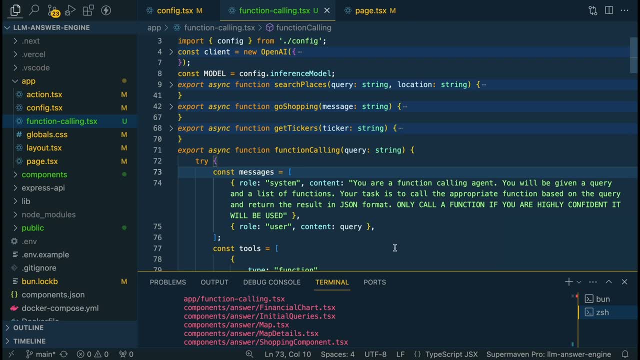 LLM. first we're just going to declare our system message here. I'm just going to specify to make it even further and hopefully more compelling to the LLM. I'm going to say: you are a function calling agent, you will be given a. 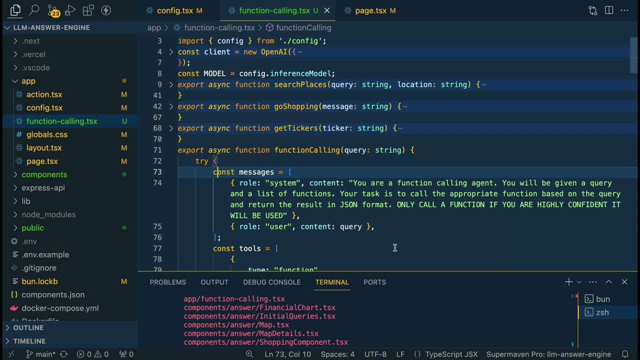 query and a list of functions. your task is to call the appropriate function based on the query and return the result in JSON format. only call a function if you are highly confident it will be used. This is the point that I get to in programming, where you just honestly have 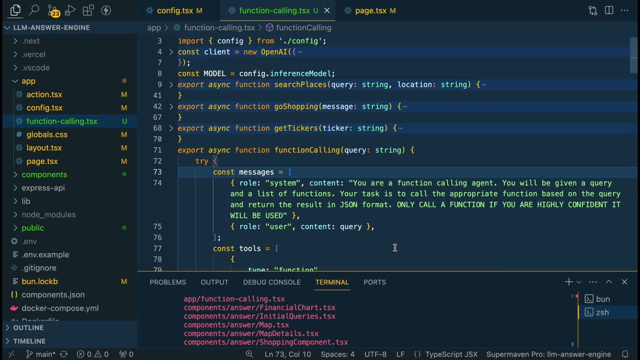 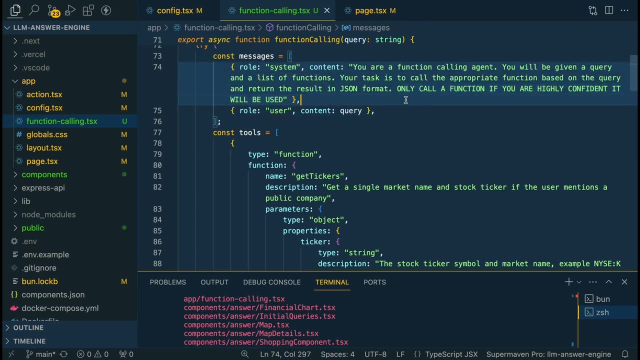 to laugh That this is what you all of a sudden have to do with interacting with these LLMs. maybe if it's uncertain that it needs to use location data. hopefully this system message is weighted a little higher, where it will recognize it and 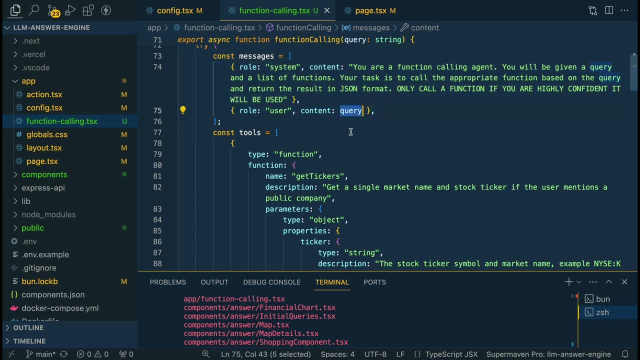 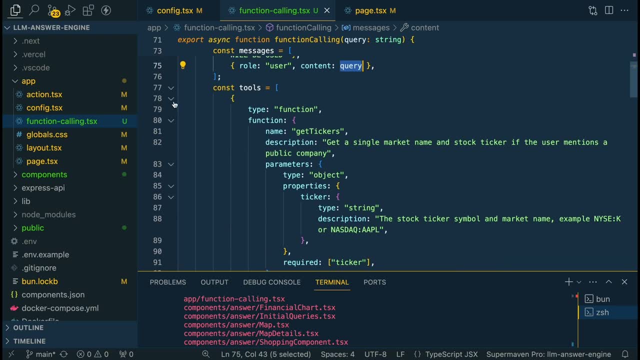 it won't call it unless it's really certain. From there we're going to be passing in the query that's going to be what in the input box on the front end, and then here is going to be where we specify the different tools that we're going to be sending in. 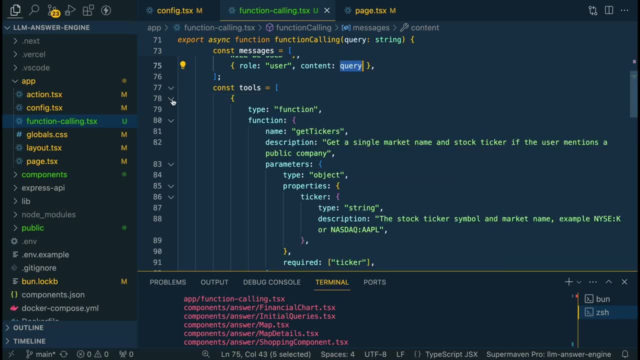 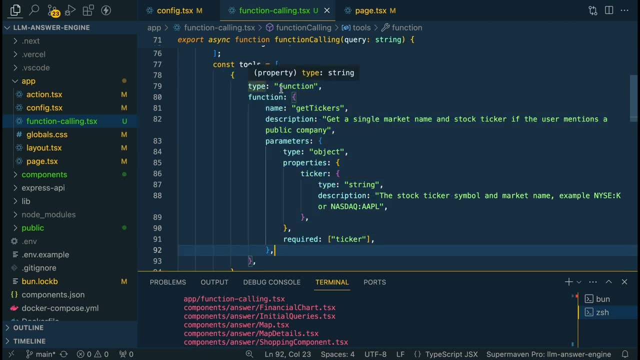 Because we have three different functions. we're going to have three different mappings within the tools here. So this is the particular schema that you have to follow to set up function calling. you're going to specify that it's a function and then, within the 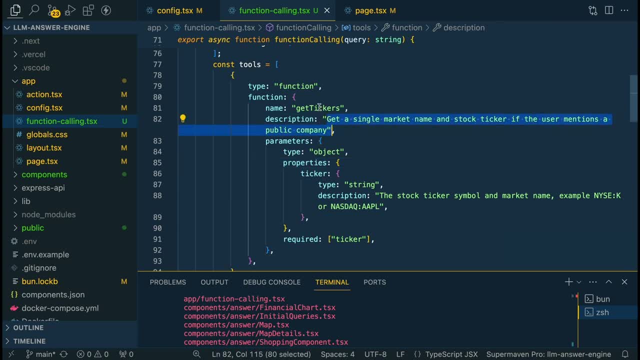 function. you're going to be describing what the function does the function name, the parameters that it has, what arguments that it has, what type of arguments that they are, whether it's a string or a number. what have you optional or required? all of that stuff is within these different tools. here you. 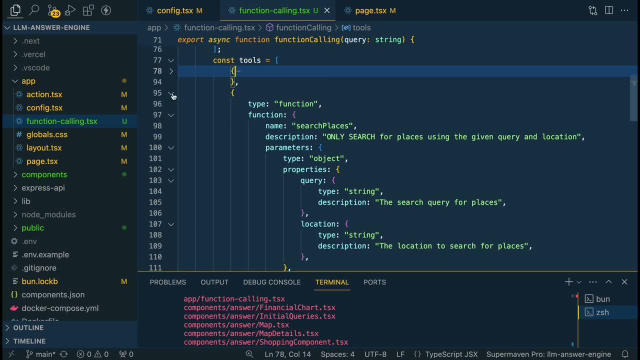 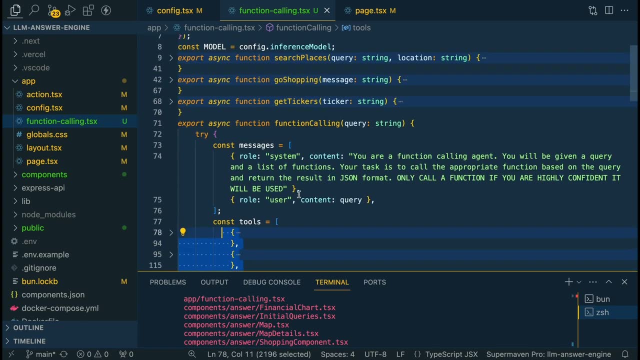 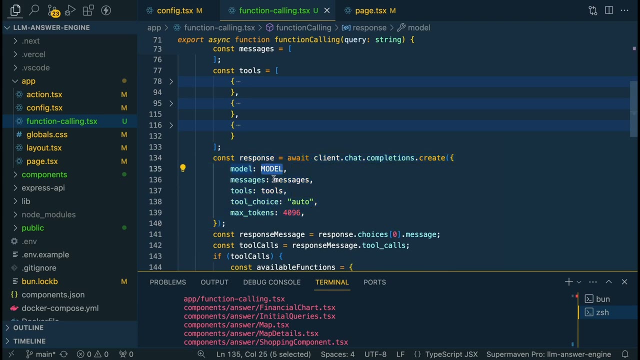 can look at these and play around with these and potentially use these and tweak them. they're all found within here and they all map to each of these individual functions here. once we have, that's going to be where we actually specify our chat completion. here we're going to be passing in the model that we have specified within. 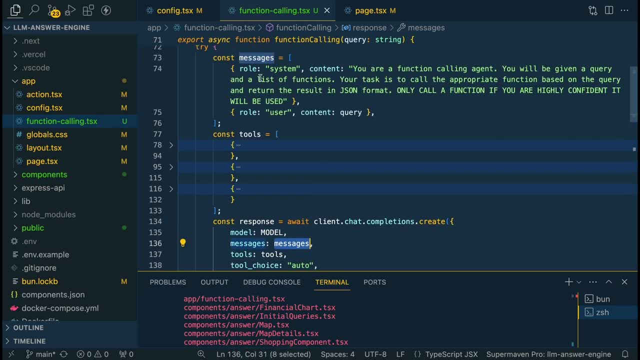 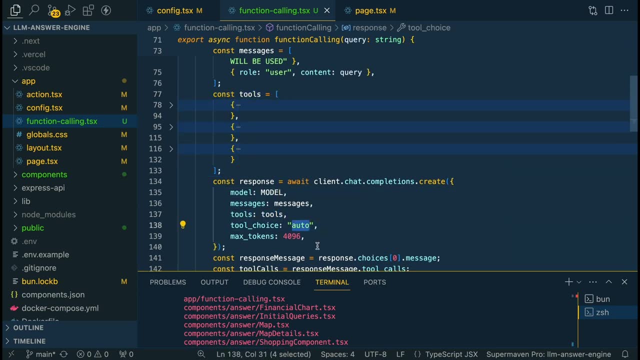 our configuration file. then we're going to be passing in the messages here that we had just declared, we're going to be specifying the tools that we just went through, And then we're going to be specifying that the tool choice is auto, And then here you can optionally choose the max token length as well. 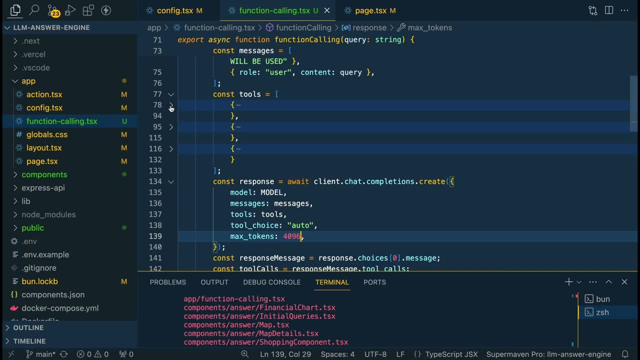 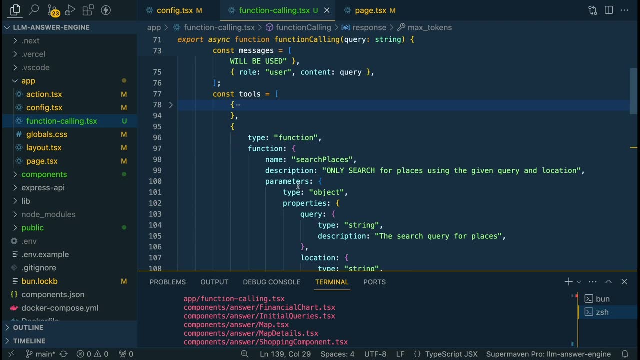 Now, one thing I found is the functions that I'm using. none of them really require long arguments. right, it's gonna be like three or four different letters. if we go to the search places, all that we're going to have is the city and the query. we have two arguments. 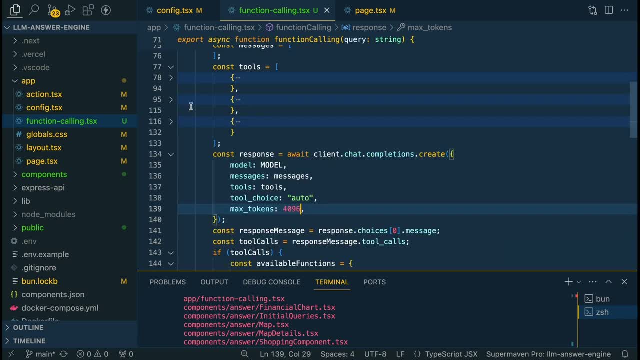 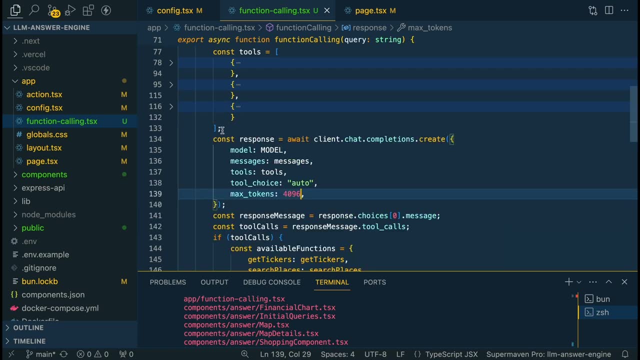 But again, we're just going to have the query and then we're going to have the location And then for the go shopping function, we're just going to have the query. So if you say Patagonia vest, it's going to say Patagonia vest. So the payload. 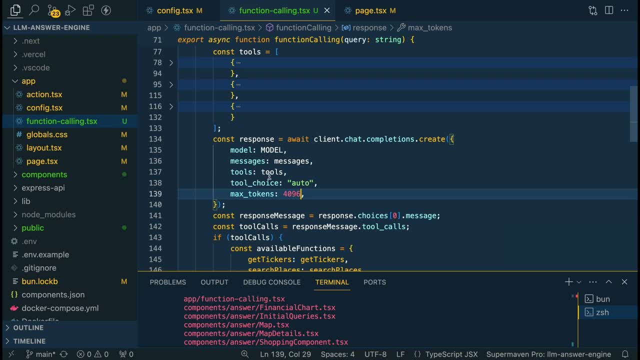 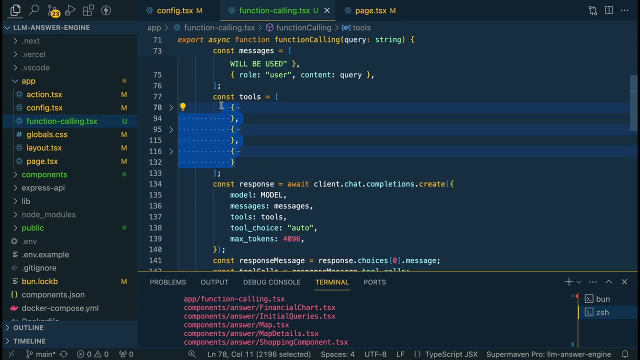 that you're actually getting back is really not that high, So there should be more than enough tokens that you need for your function invocations, unless you're doing something really adventurous where you have a ton of different things here. The next one we're. 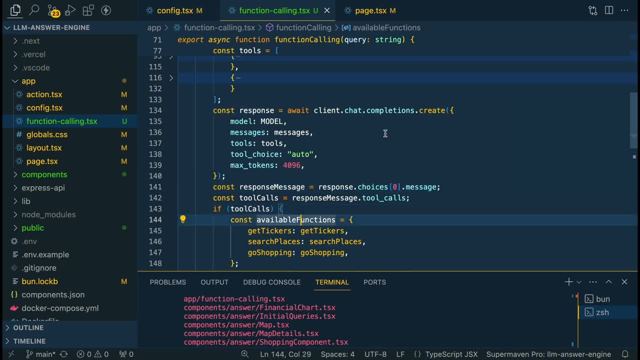 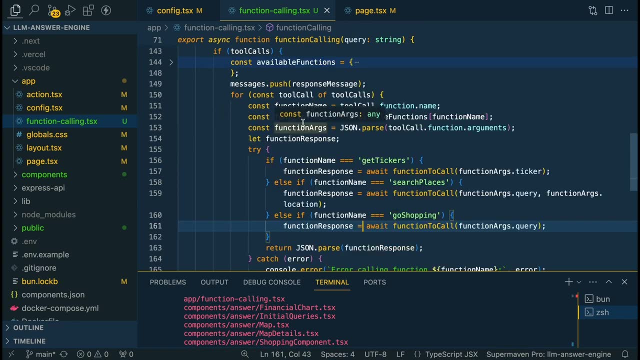 going to be setting up is, once we have that response message, we're going to have it within this response message variable, Now within the tool calls. essentially, what we're going to be doing is we're going to be looping through the different tool calls that were detected. 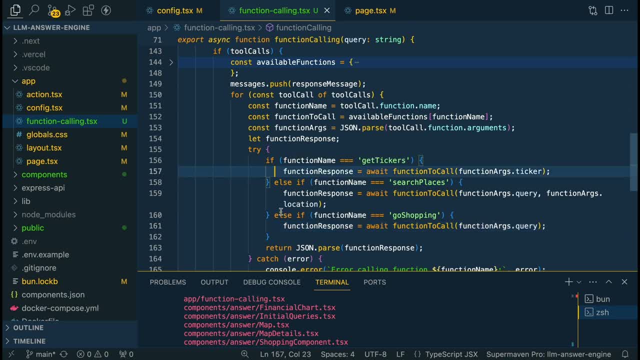 if there are multiple, and then in here we're just going to go through and see which ones were detected In this application, like I mentioned, I'm only really expecting to call one function, But you could set it up in a way where you have multiple functions that are being called. 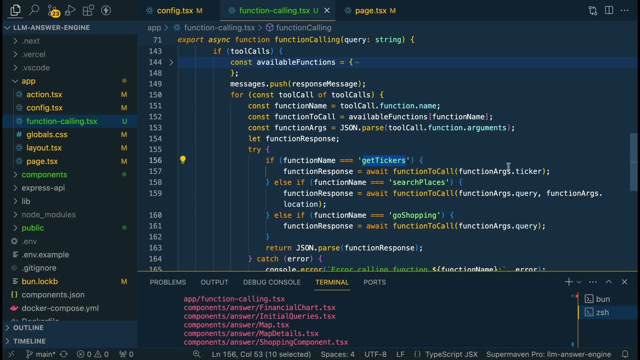 So here, if it detects get tickers, we're just going to go ahead, call that function with the payload that we got back from the LLM. So this would be like something like the L for Apple sticker. if it search places, we're going to have the query and the location. 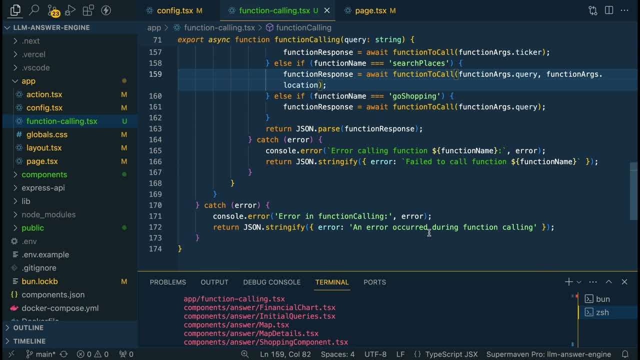 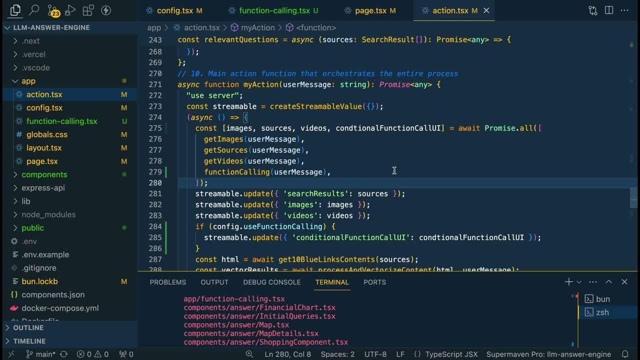 I've made a couple tweaks to the Action notes x And basically all that I've done is within our promise where we're concurrently getting the images, sources' videos. Now we're also going to be doing the function calling where you could also take out and move it. 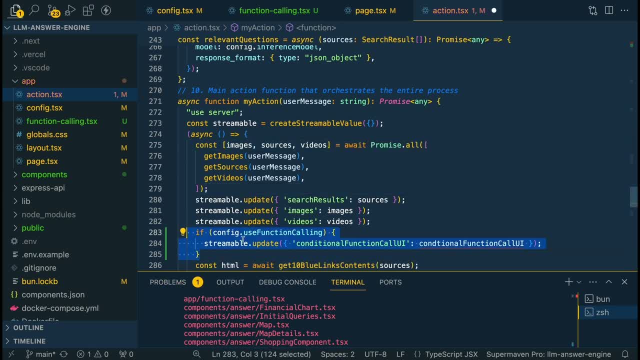 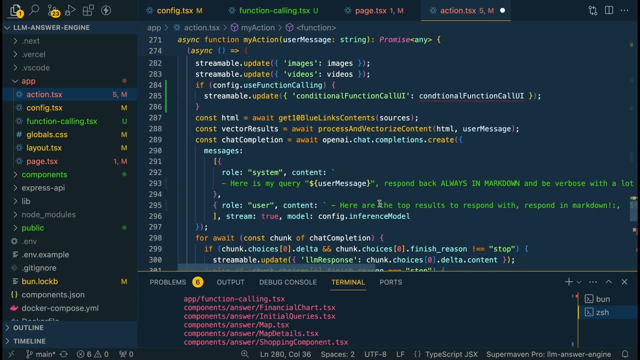 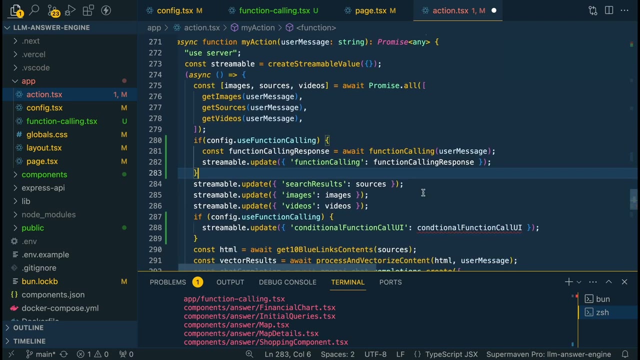 below and do something like I have within the stream update here. So we could say something like: if config dot use function calling, and then within that we could just specify: we want the function calling response to be the user message, And then we could have this. 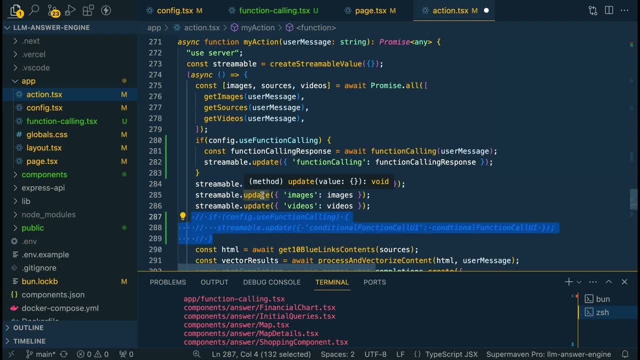 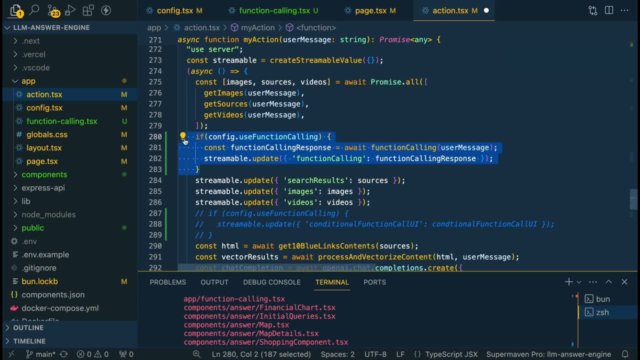 streamable response there if we'd like, And then that way it's just adjacent. but you are going to be waiting longer if you have it set up like this, But that way the whole configuration can just be wrapped. you can turn it on, So you have that flexibility if you'd like. but I'm just going. 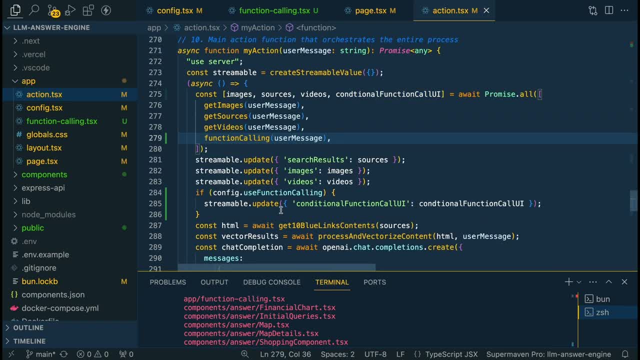 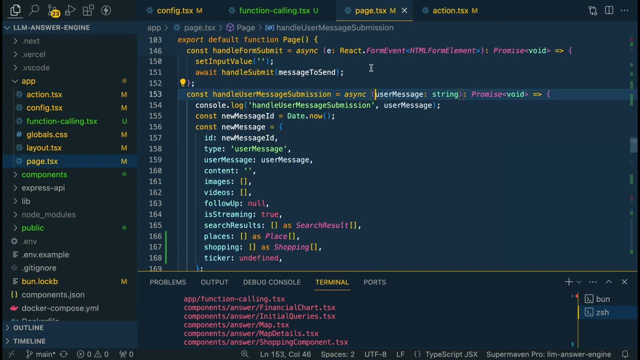 to move it back to the way that I have it and then just save it out here So you can play around with these a little bit, depending on what you'd like to see or how you'd like to have it configured Then within the page. I'm going to go through this relatively quickly, But the best way. 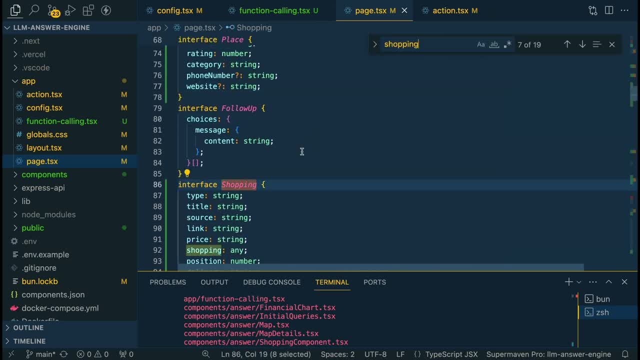 to go through and see what I did to set this up is if we look at some of the new components, the shopping component for instance. So you see all of the different types that we have for the shopping component. Now you can just go through and you can search shopping on the new. 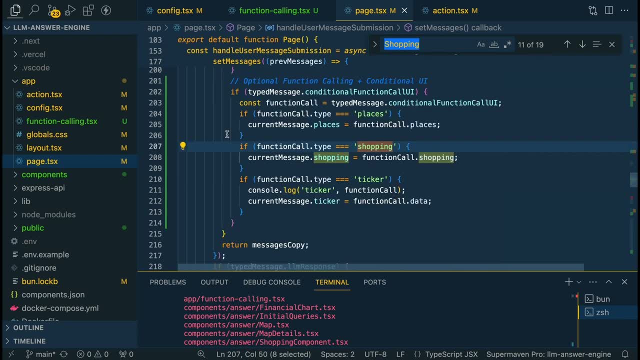 message. we have these new keys. the main portion on how it determines where in the UI is going to go is we have this similar structure that we had in the previous video on how we determine where the different things go. here we have this setup, So if it detects that there's conditional function, 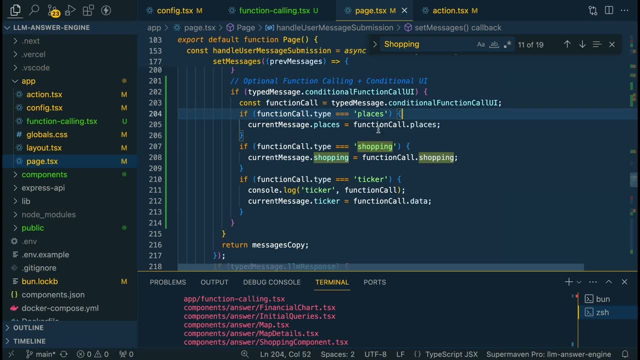 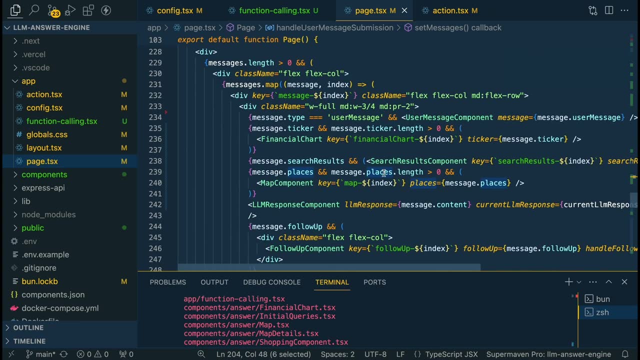 call UI. we're going to go ahead and parse that And we're going to look for the different keys. So, whether it's places, shopping or ticker, it's going to go ahead. put it within state, within our application for places, within that grouping of messages. we're just going to push it on the. 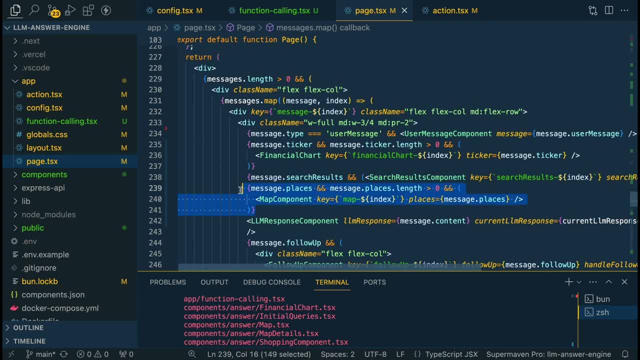 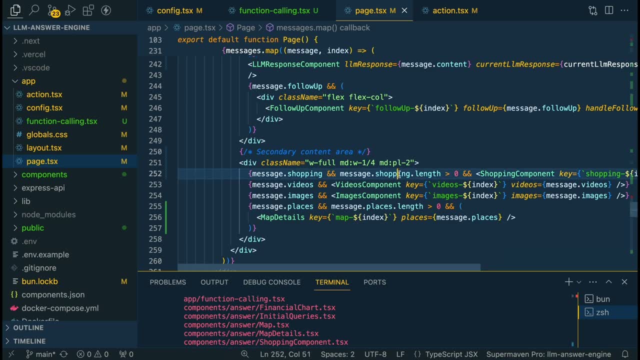 places key And then, with our messages map, we're going to go ahead and put it on the places key. We're going to pass in the props of places into our map component Or, for instance, if it's our shopping component, we're passing the props into our shopping component. And the way that I have 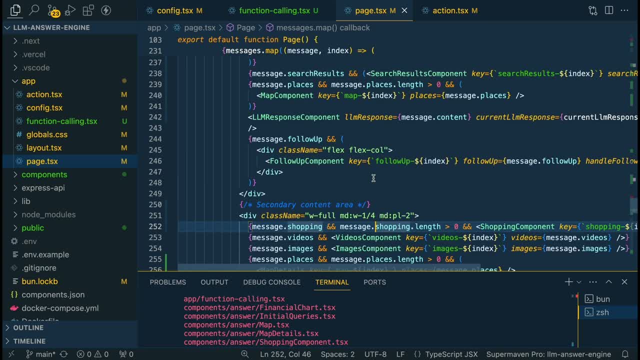 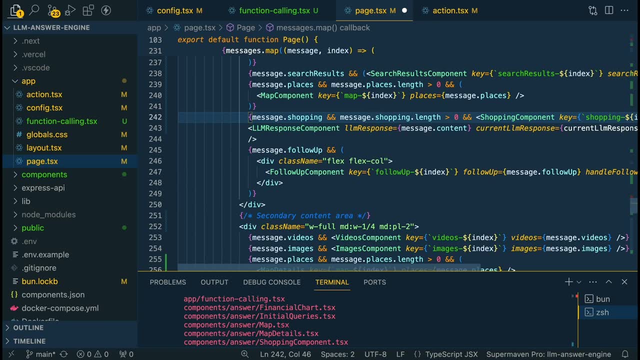 this setup is: you can really move these around. So say, if you want the shopping component on the secondary content area or the sidebar, you can have it there. Or if you want it right at the top results, you can go ahead and save it up there. you can really play around with these things. 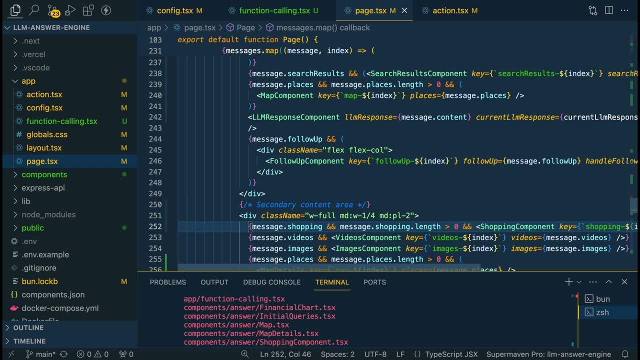 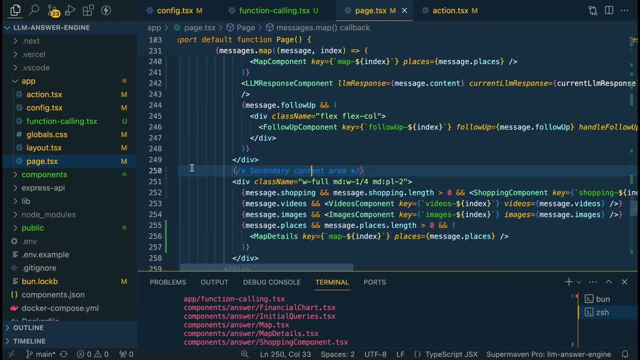 There's like Lego blocks. you can move them around however you want. They're set up in a way where if you move them through, they're just not going to render. So that's pretty much the main changes that I made to the page dot TSX And then just for the actual components themselves, you see, within my 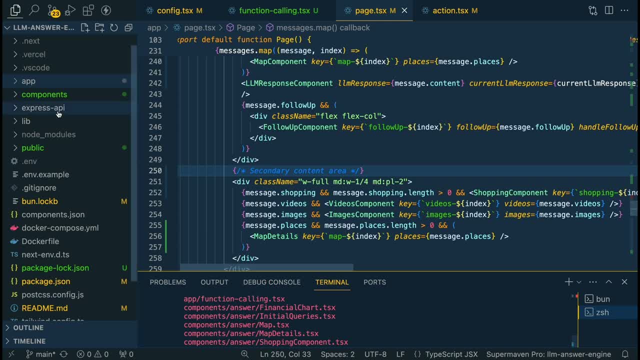 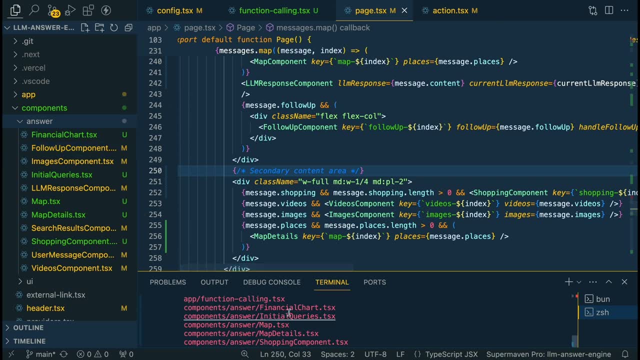 terminal. here you see all of the new files that I have here within the project. So we have a handful of new components here, So I have them in the answer directory, just like I have the other ones. So within here we have five new components. we have a financial chart from trading view. we have 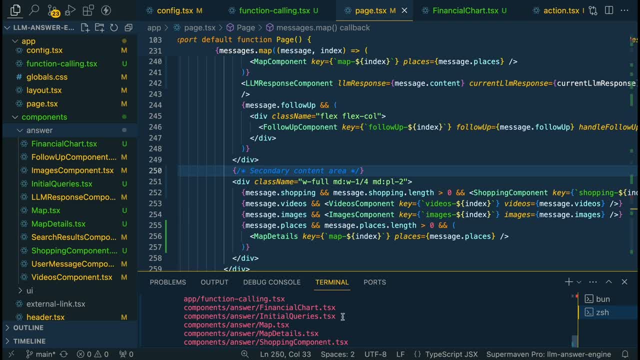 the initial query, which is the initial queries that we have on the screen Here. you saw in the original example, we have our map, we have our map details, where it shows the details of the location on the right hand side there, And then we have our shopping component. 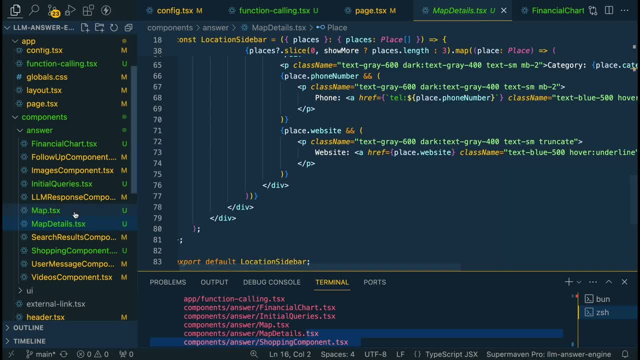 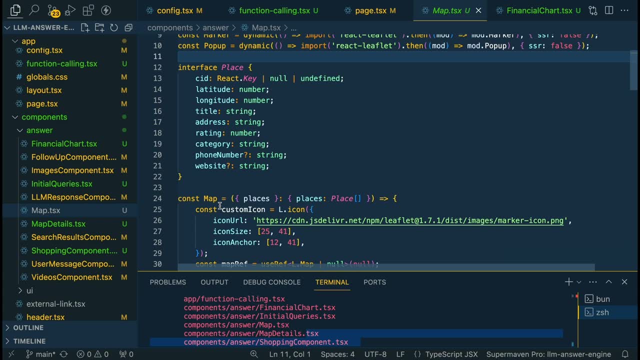 take a look at how they're set up. Some of them are more simple than others And some of them are just interesting to use, But hopefully it just serves as an example of different things that you can add within the project. So if you're interested and you have some ideas and you want to take a stab, 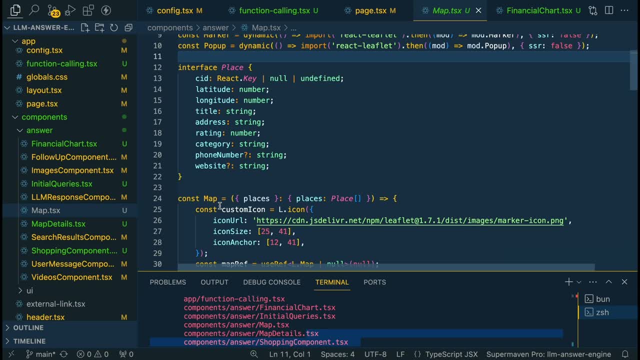 at throwing in some interesting components within the project. make a pull request, submit an issue time I'll try and add some of the features that people have requested, But otherwise that's pretty much it. If you found this video useful, please comment, share and subscribe, and otherwise until.